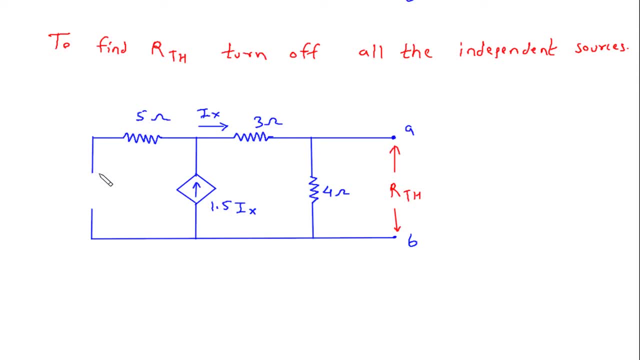 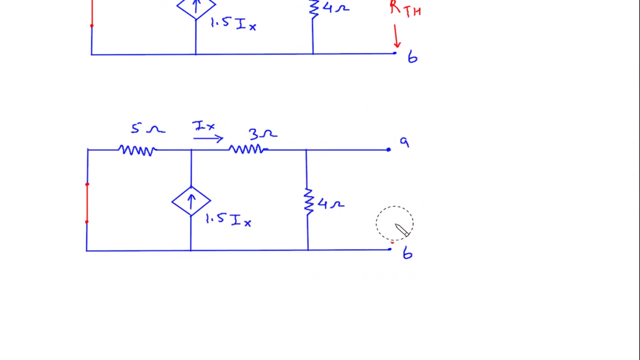 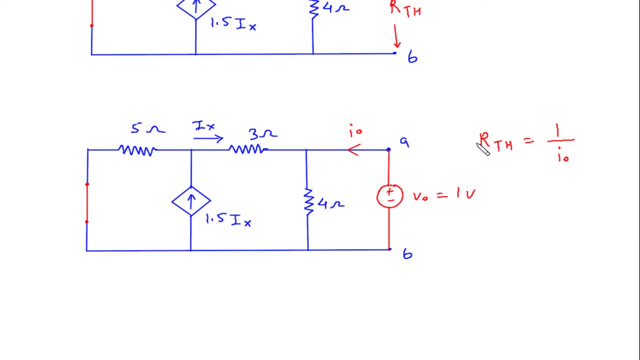 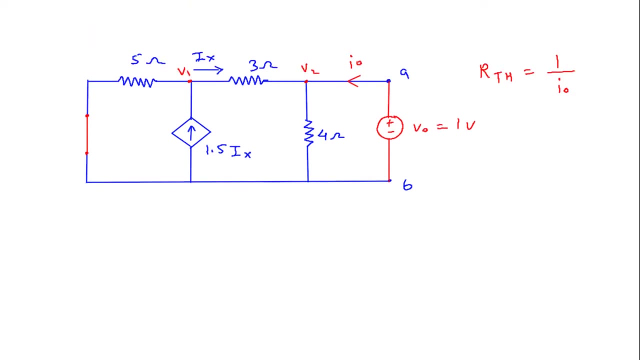 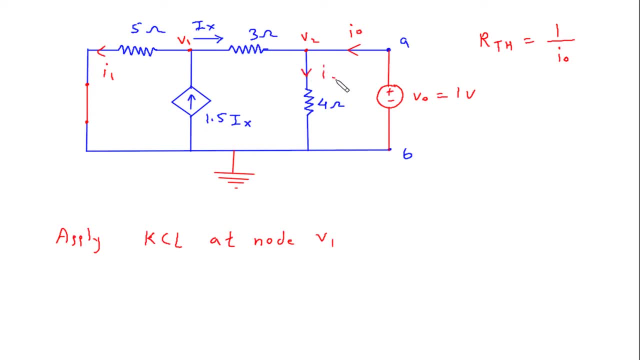 current IO. this is current i2. so apply KCL at node v1. so entering current at this node is 1.5 ix. leaving current is equal to leaving current is ix Plus ix plus i1, so this will be 1.5 ix minus ix minus i1 is equal to 0.. 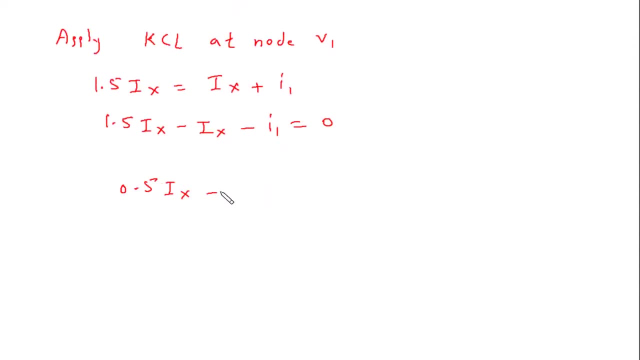 So this will be: 0.5 ix minus i1 is equal to 0. now 0.5 ix is v1 minus v2 by 3. v1 minus v2 by 3 minus i1 is this: i1 is v1 minus 0 by 5. v1 minus 0 by 5 is: 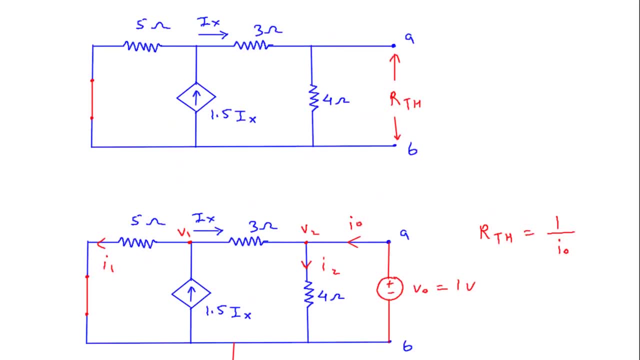 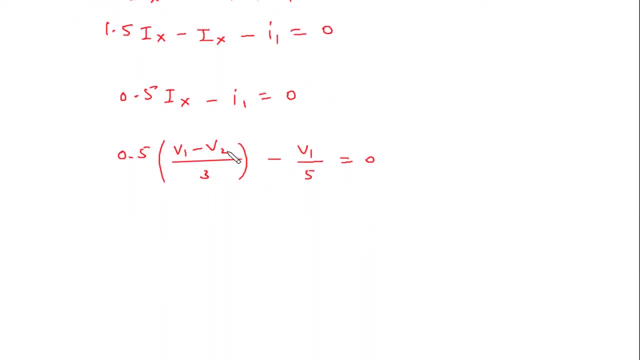 equal to zero. So this is v1 minus 0 by 5.. So this will be 0.5 ix. V1 by 3 minus 0.5. V2 by 3 minus V1 by 5 is equal to 0.. 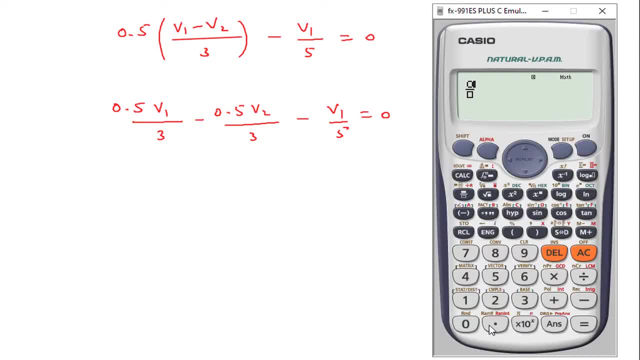 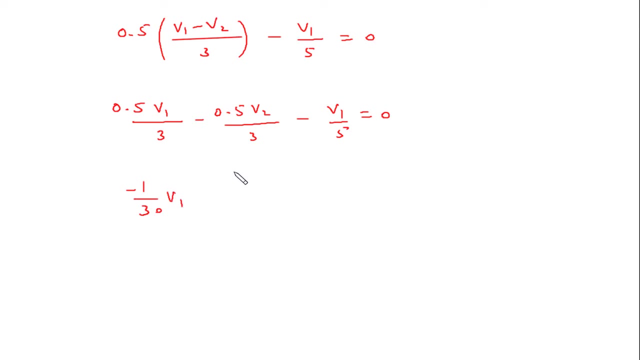 So this will be 0.5 by 3 minus 1 by 5 minus 1 by 30, V1 minus 0.5 by 3, V2 is equal to 0. Let's say this is equation number 1.. 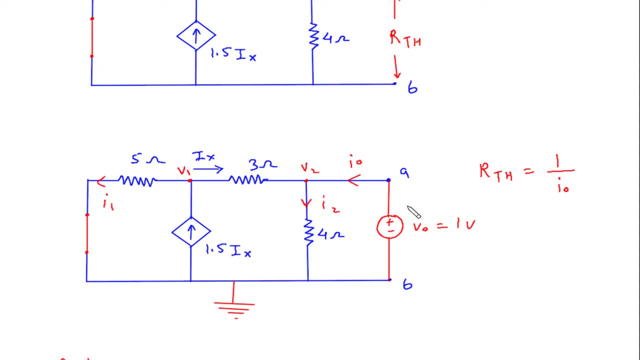 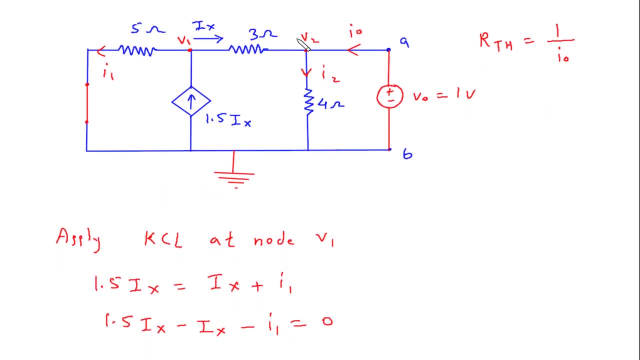 Now we will apply KCL at node 2.. But as we can see that V2 is equal to V2 is equal to Vo and Vo is 1 volt, So this will be 1 by minus 1, by 30, minus 0.5, by 3 into V2, V2 is 1.. 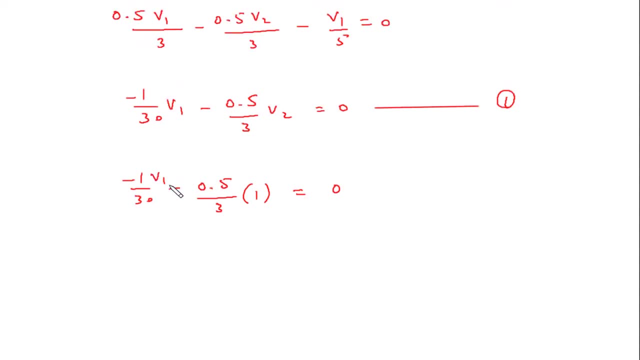 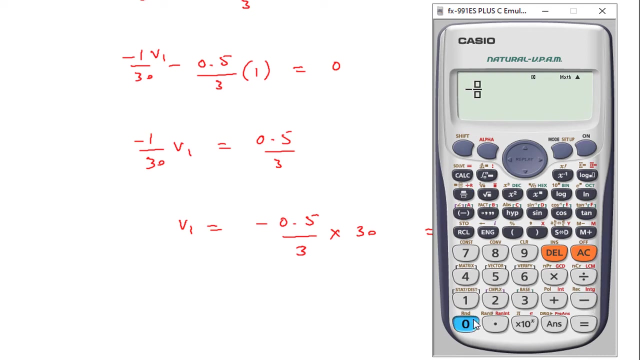 So from this we can calculate: This is V1 minus 1 by 30. V1 is equal to 0.5 by 3.. So this will be: V1 is equal to minus 0.5 by 3 into 30, minus 0.5 by 3 into 30.. 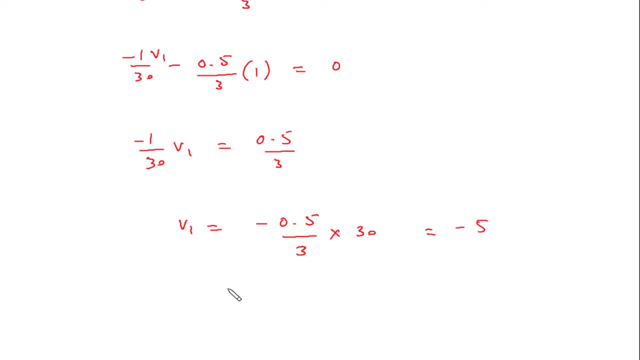 So this is minus 5.. V1 is equal to minus 5.. What we have to find? We have to find this IO. Now, IO is equal to when we apply KCL at node V2.. Then entering current is IX Plus IO. IX plus IO is equal to I2.. 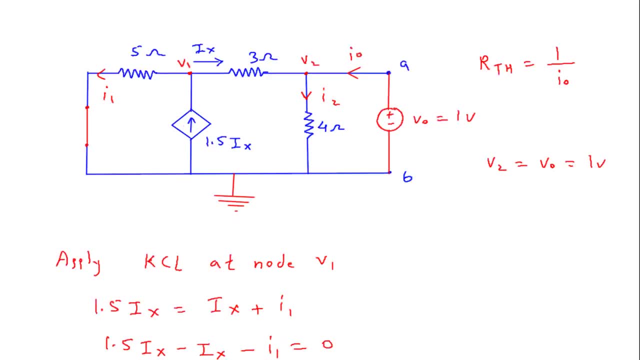 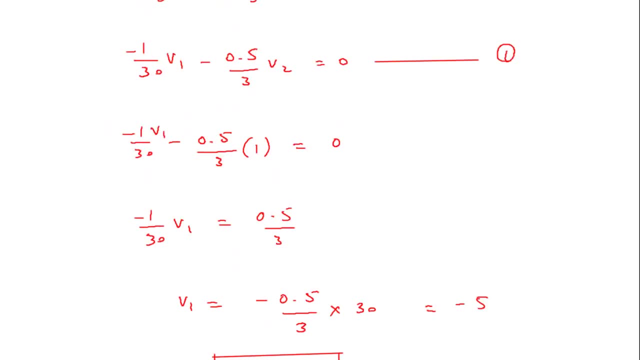 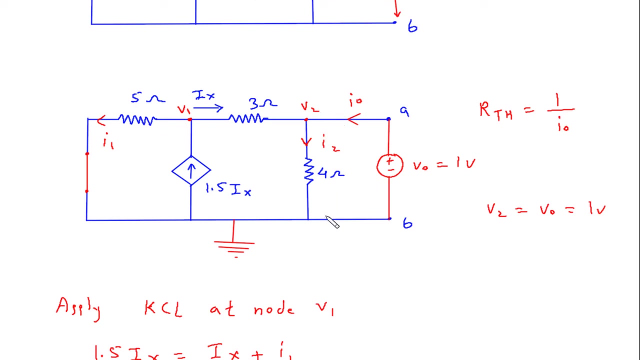 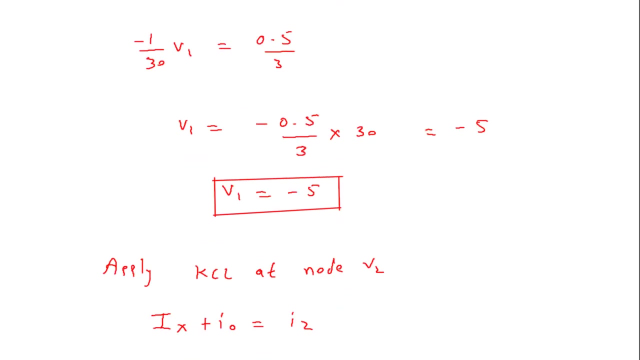 So IX is V1 minus V2 by 3. V1 minus V2 by 3 plus IO is equal to I2 is 0.5 by 3.. So this will be V2 minus 0 by 4.. So this will be: we have the value of V1.. 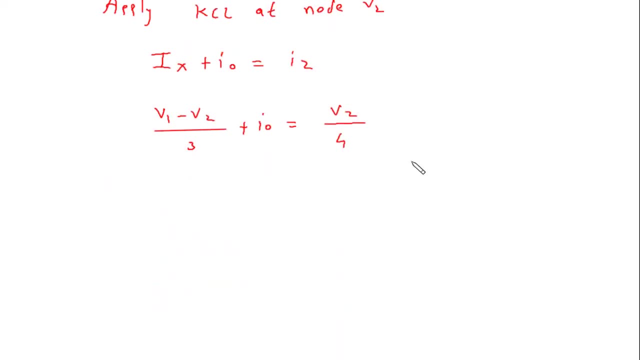 V1 is minus 5 minus 5 minus V2 is V2 is 1 volt. So 1 by 3 plus IO is equal to V2 is 1 by 4.. So from this, from this, IO is equal to 1 by 4. this will be minus minus 5 minus 1 by 3. 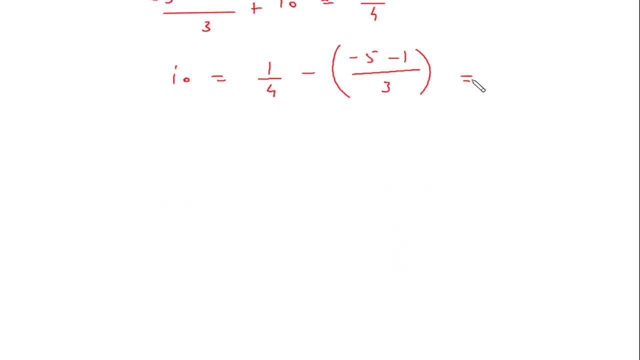 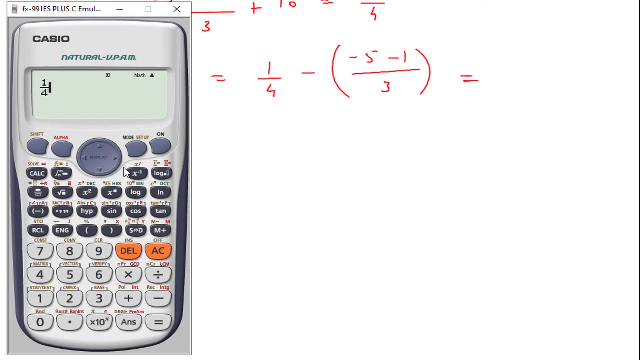 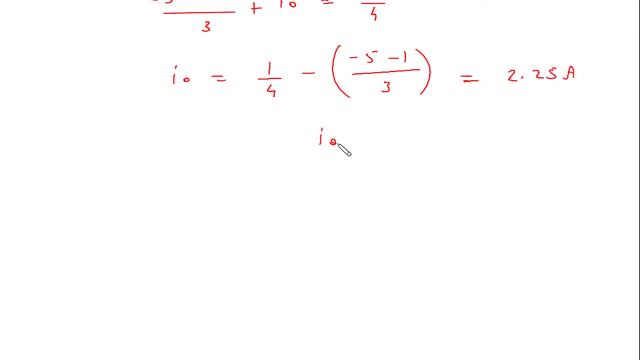 1 by 4 minus minus 5 minus 1, 3, 2.25 Ampere. IO is equal to 2.25 Ampere. Now from this we can find the value of Rth. Rth is equal to 1 by IO. 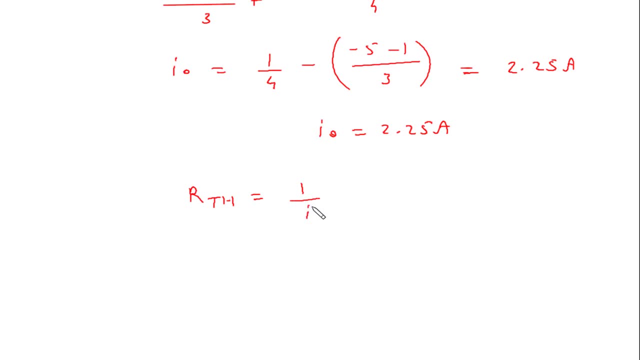 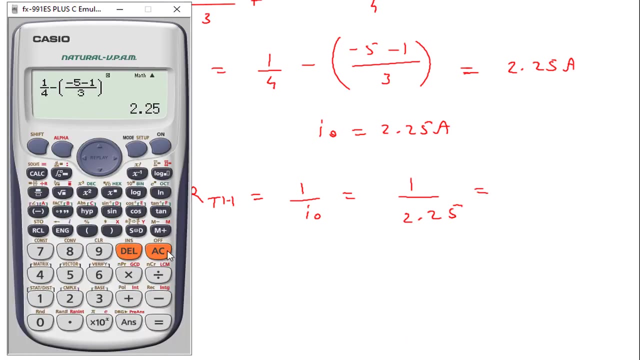 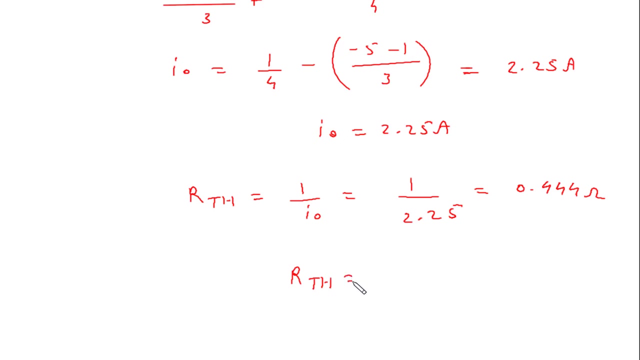 Rth is equal to 1 by IO, so 1 by 2.25. 1 by 2.25 is equal to 0.444 Ohm. Therefore Rth is equal to 0.444 Ohm. To find Vth, Let's say this is node with V1. 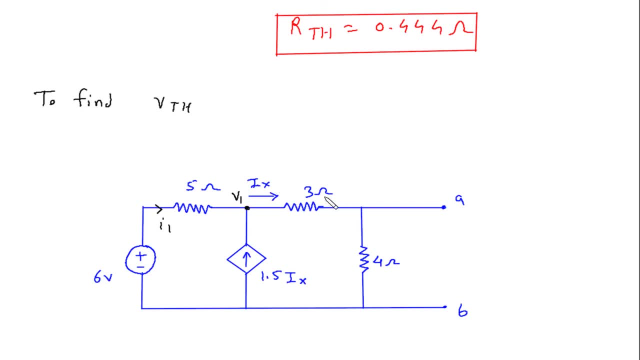 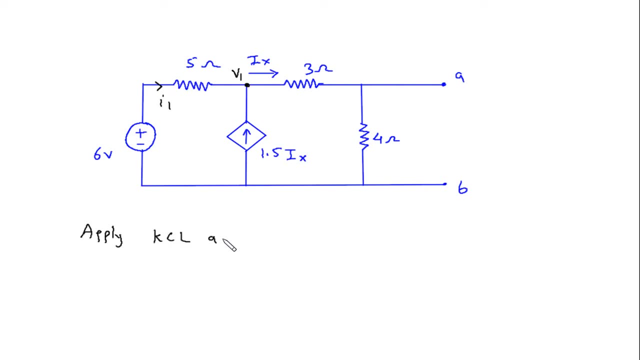 Let's assume this is current I1, this is current Ix, So apply KCL at node v1. So entering current node is i1 plus Ix. 1.5Ix Is equal to leaving current is i x, so this will be I1 plus 1.5I x. 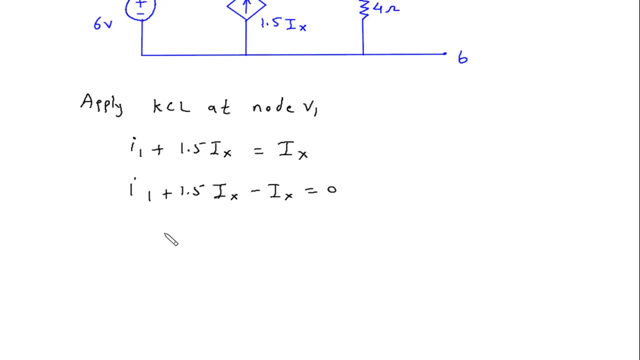 minus Ix is equal to zero. Now this will be I1 plus 0.5. Ix is equal to 0.. So I1 is 6 minus V1 by 5, 6 minus V1 by 5 plus 0.5 Ix is this? Ix is, let's say this: 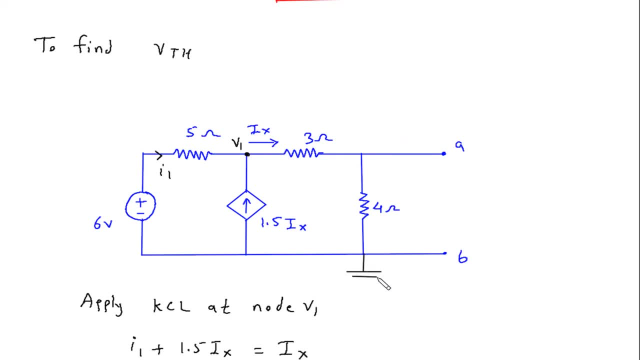 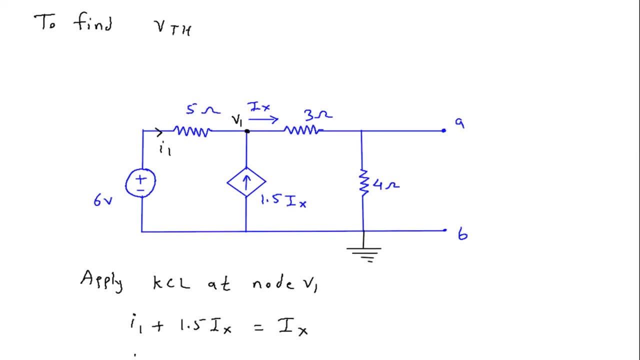 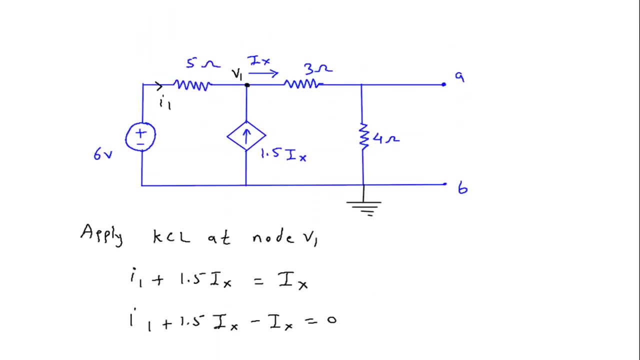 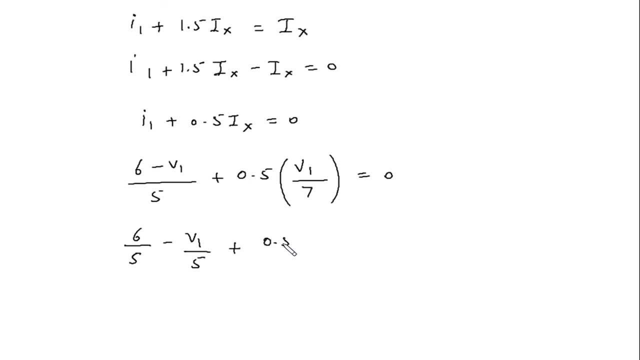 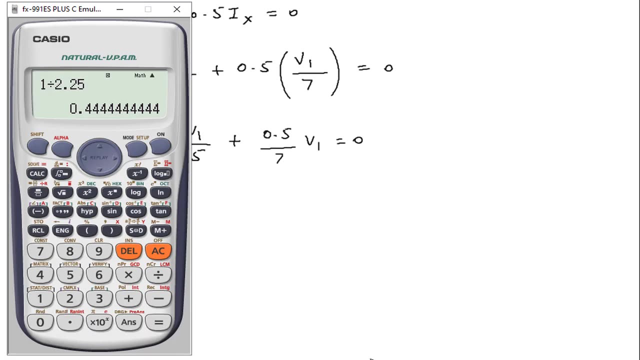 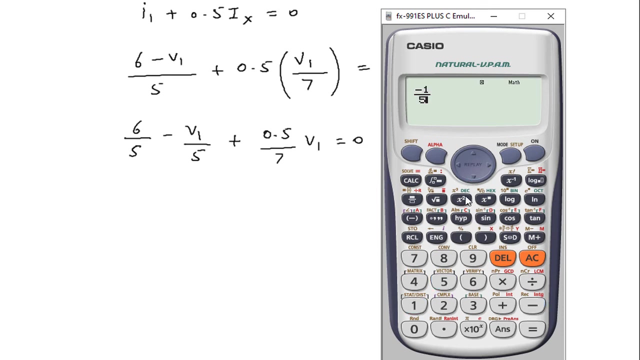 5, plus 0.5 by 7, V1 is equal to 0.. So this will be minus 1 by 5 plus 0.5 by 7, plus 0.5 by 8, minus V1 by 10 plus 0.5 by 10. 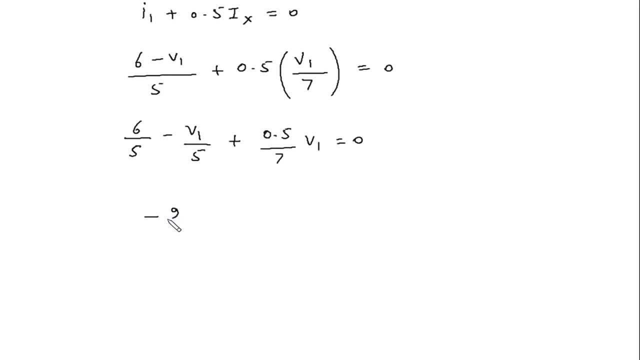 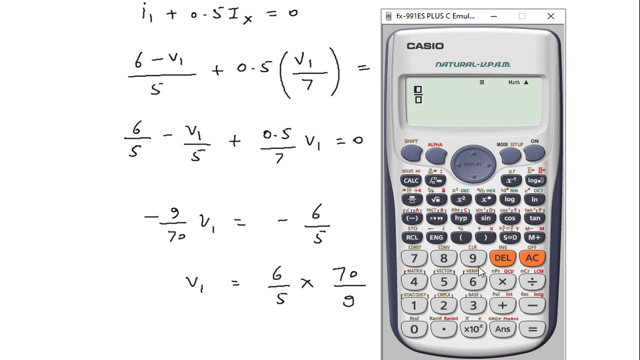 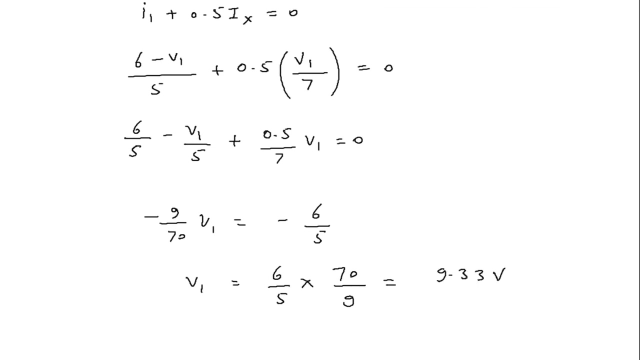 minus 9 by 70. V1 is equal to minus 6 by 5, so this will be: V1 is equal to this minus and this minus will get cancelled. So 6 by 5 into 70 by 9.. 6 by 5 into 70 by 9. 9.33 volt. 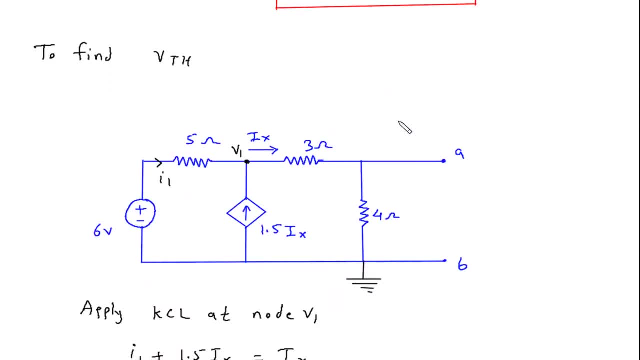 is the value of V1.. Now we have the value of V1.. So Ix is equal to V1 minus 0 by 7.. Ix is equal to V1 minus 0 by 7.. So V1 is 9.33 by.